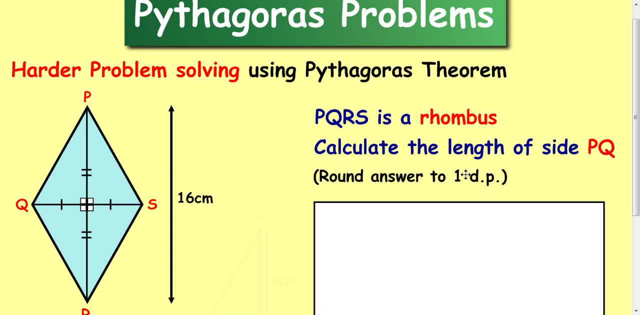 in the marking scheme. So with Pythagoras we're looking for right angle triangles. So if you're trying to work out PQ, you can see a right angle triangle here, This portion here. if I was to colour that in just roughly, There's a right angle triangle in there. So the easiest way to work out PQ is to actually 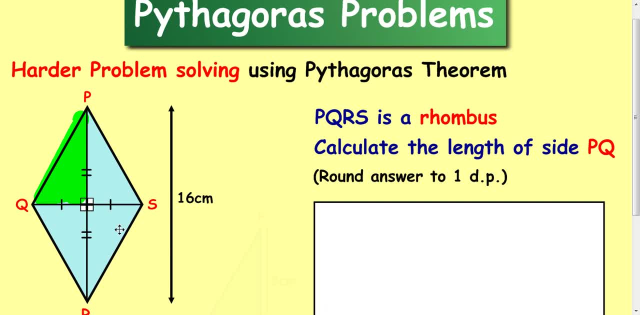 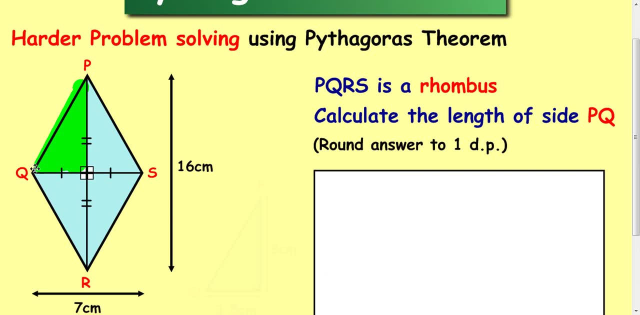 take that triangle out and draw it. So the things we need in the right angle triangle are we need two sides to then work out PQ. So I need to think if I can get this side in the bottom. So all the way across is 7cm and these wee two lines here means that that 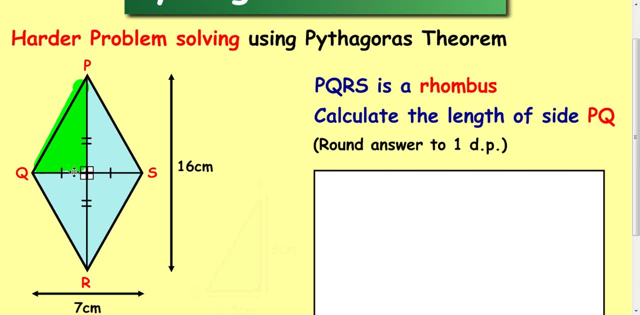 line and that line are the same length. So if you half 7 you'll get the bottom bit of this right angle triangle and that's 3.5.. And the same thing with this bit up and down the way. This diagonal of the rhombus is 16cm. These two wee lines and these two wee lines. 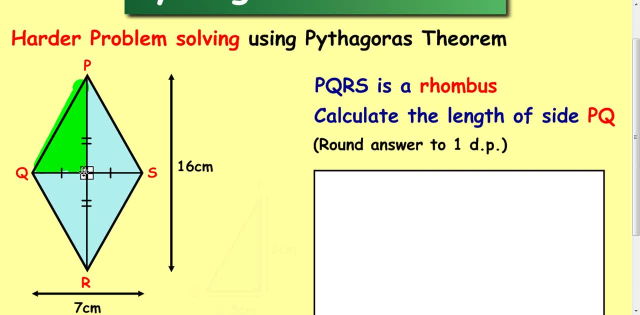 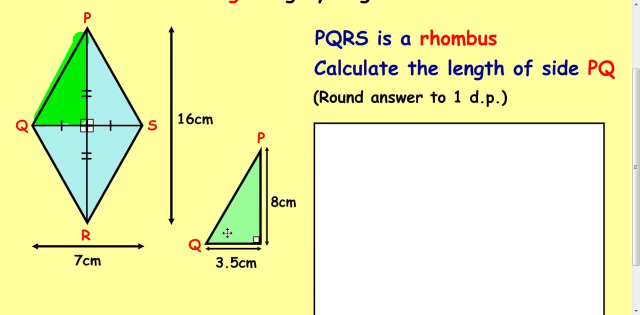 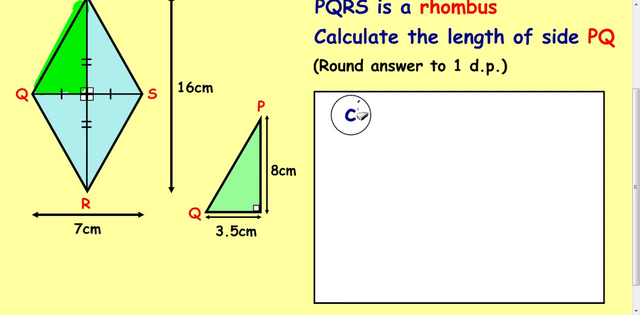 mean these are exactly the same size. So if you half 16 you'll get the height. So drawing the wee triangle out, you will get this idea here And then we can just work out PQ doing a straightforward Pythagoras question. So PQ squared, or C squared, equals A squared plus. 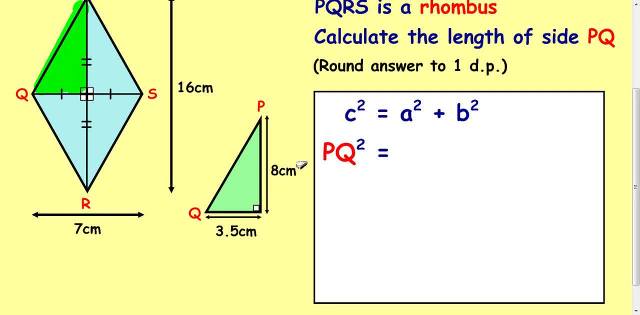 B squared. Then we can go into: PQ squared equals 8 squared plus 3.5 or 3.5 squared plus 8 squared, It doesn't matter which way round you do it, PQ squared is equal. to put that into your calculator and get this coming out: 64 and 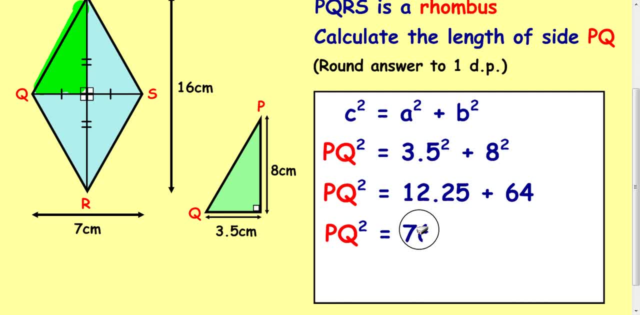 12.25.. Add them together to get 76.25.. And then, finally, to get PQ, which was the question, you square root 76.25 and you get 8.7.. Now, I haven't done so here. What I would advise: 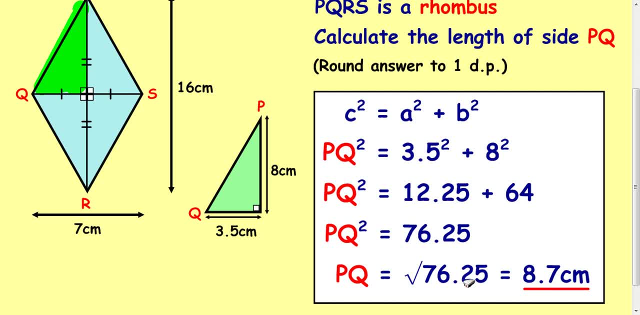 you to do is get your unrounded answer and then write your rounded answer underneath. It's going to do it. Now you have a nice round pass line like this. Ok, now we are going to draw from square root. Our round pass line here has a point. So we are going to go to square root and our square root is then going to be going to be going under square root. Here we have our round pass line. We are going to start off with the square root, So first we have to add our square root. And then we are going to add our round pass, line X. Now I'm going to go down and add counter straight to square root, So the line we're going to have to do is going to be $1.. Now we also need to add our real square root.